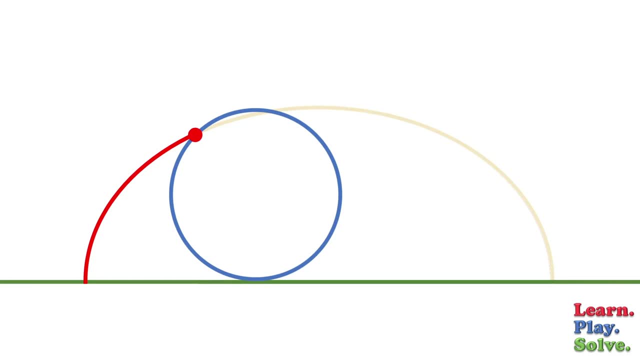 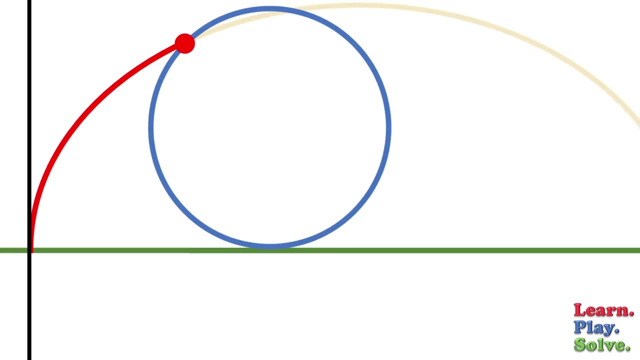 to visualize the relationships between the variables in play here. Let's imagine this on the Cartesian plane, with the cycloid starting at the y-axis, The point on the circle that is tracing out the curve will be xy. This is our primary focus. We want to find the 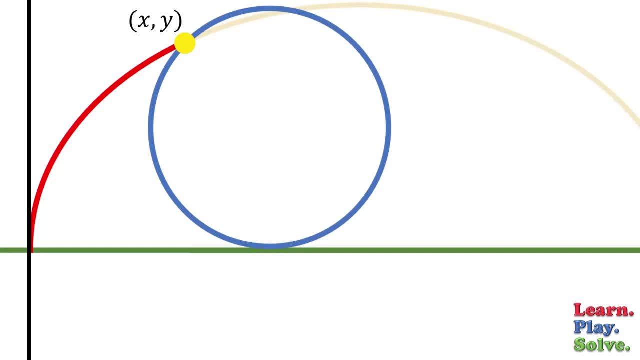 relationship between x and y that describes this curve. To do that, let's start by using the gradient. First, we want to determine the radius of the circle that generates the cycloid. That will always be the distance from the center of the circle to the ground. 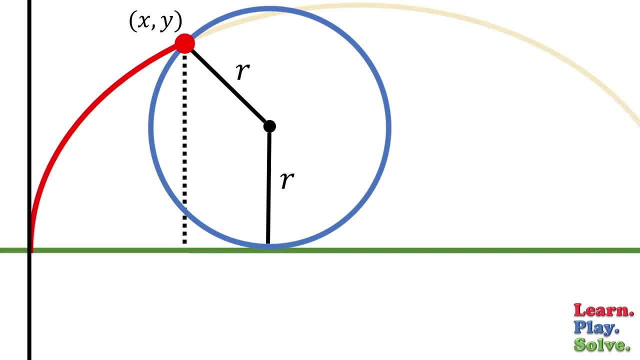 Let's also draw a line straight down from our point xy. This represents the height of the point at any given moment, which is simply the y-coordinate, And the distance to that line from the y-axis is the x-coordinate. If we make a right triangle here and let the base of the triangle be A, then this line 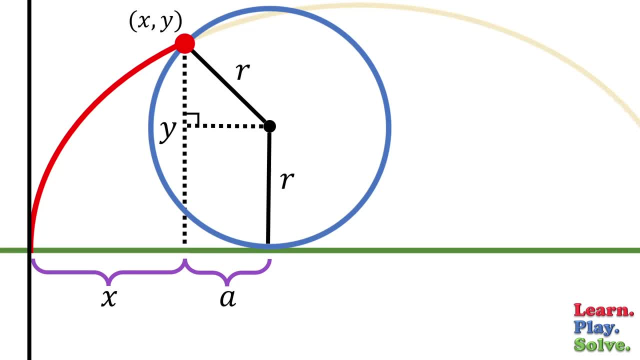 segment must also be A. Therefore we can call the total distance. the circle has rolled x plus a. This distance must also be equal to the arc length of the circle, And the arc length of any circle is equal to the measure of the angle that traces out. 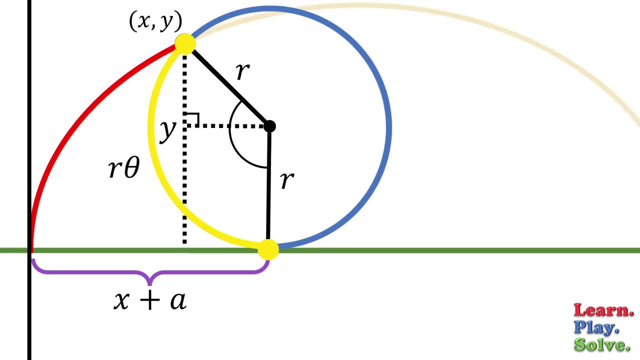 that arc times the radius of that same circle. So this distance is r theta, which means x plus a is r theta, And if we solve for x, we get x equals r? theta minus a. For y we can break it into two smaller segments, one of which we know is equal to the radius. 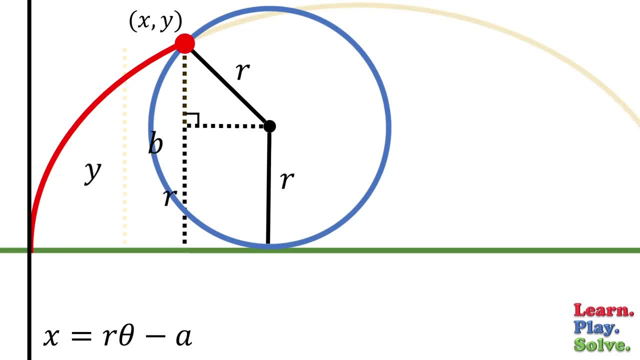 and the other one. let's call it b for now. So y is equal to b plus r or r plus b. We now have a set of parametric equations. The parameter in this case is theta. But what about a and b? 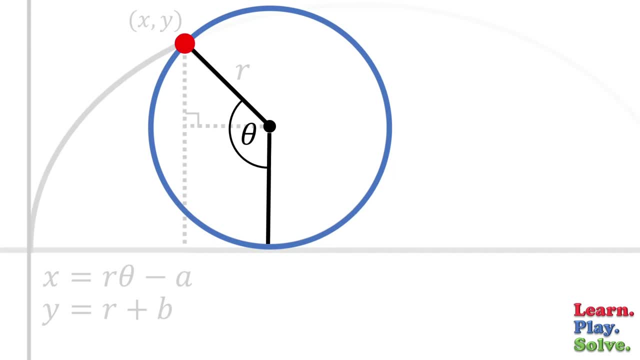 Remember that the angle the circle has rotated up to this point is theta. This part is a right angle or pi over 2 radians. So if we subtract pi over 2 from theta, that will be the angle inside this triangle. Also, remember we called the legs of this triangle a and b. 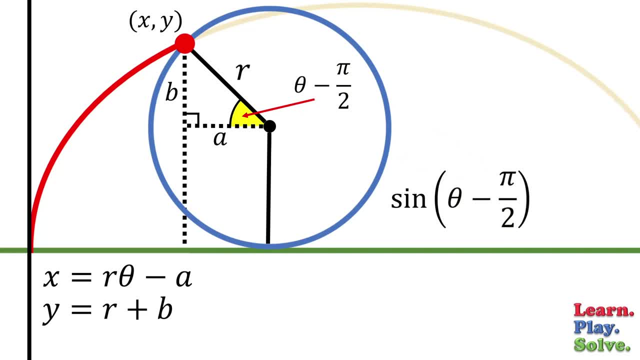 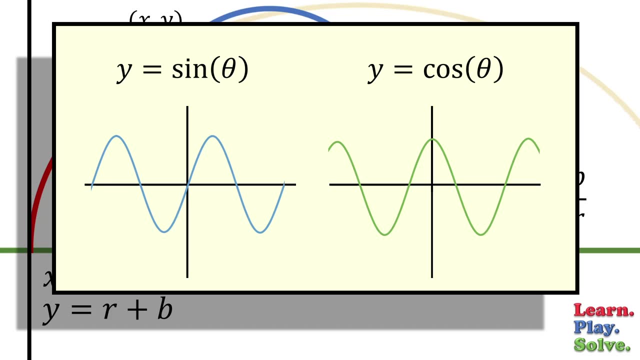 The sine of the angle, theta minus pi over 2, is the opposite side over the hypotenuse, which is b over r. We can simplify this trigonometric function. Look at these two graphs, If you notice. for the sine function, if you subtract pi over 2 from theta, it shifts the. 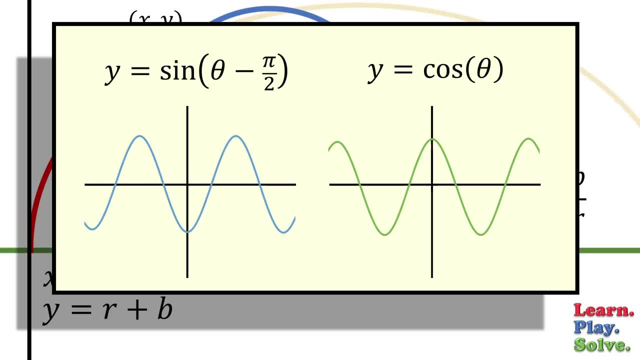 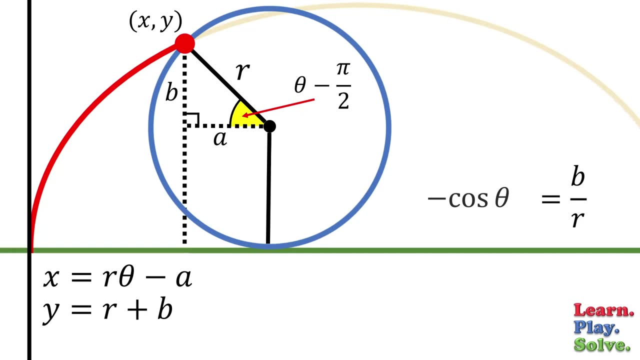 graph over like this: This is identical to what would happen if we flipped the cosine function vertically. So sine of theta minus pi over 2 is equal to negative cosine theta. That gives us a simpler equation. We can solve for b by multiplying by r. 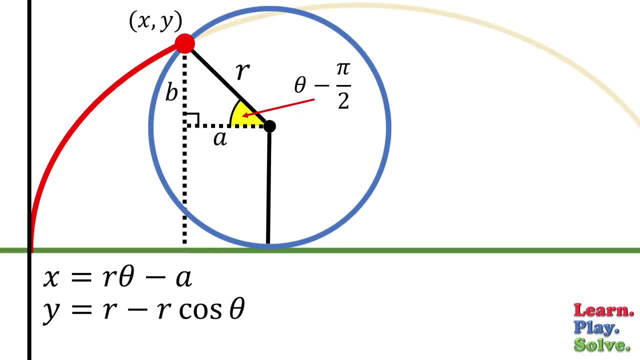 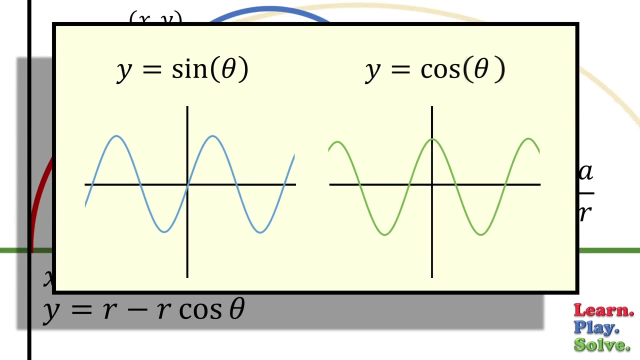 Plug that in and we have y equals r minus r, cosine theta. Now let's take the cosine of our angle. Cosine is adjacent over hypotenuse, which is a over r. Again, we can simplify this If we change the cosine function by subtracting pi over 2, it'll shift it like this: 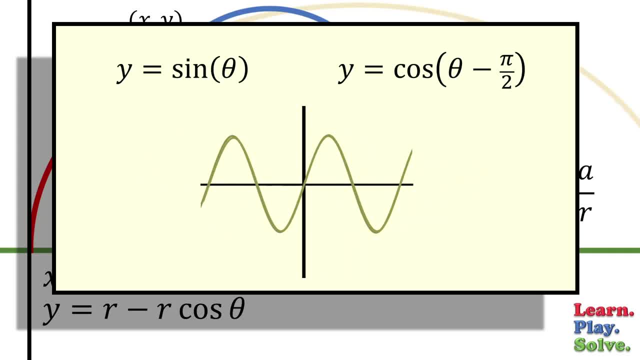 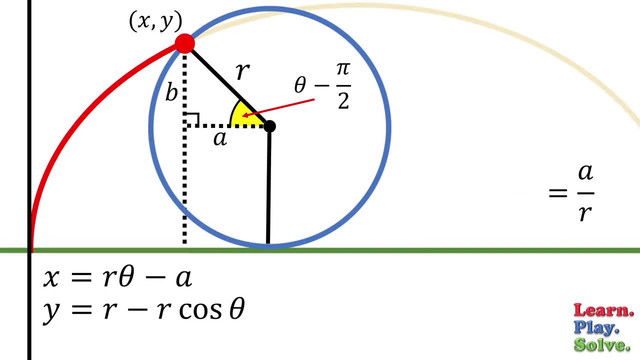 This is identical to the sine function as it is Now. let's try this again. So the sine of theta is equal to cosine of theta minus pi over 2.. So this simplifies to sine theta equals a over r. Solve for a and plug this in, and here we go. 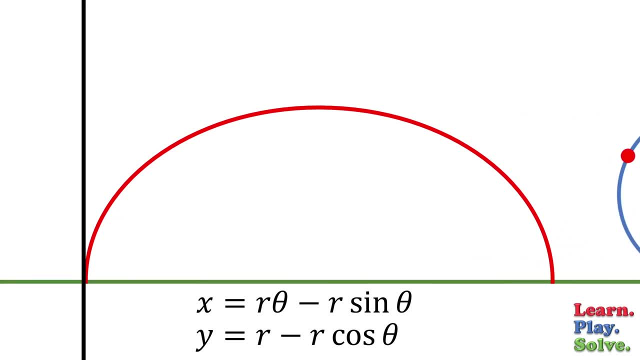 The parametric equations for a cycloid. We could plug in any radius to change the size of the curve. You might be wondering: is there just one equation for a cycloid? And the answer is yes. Although it's not an explicit equation, we can get it pretty close. 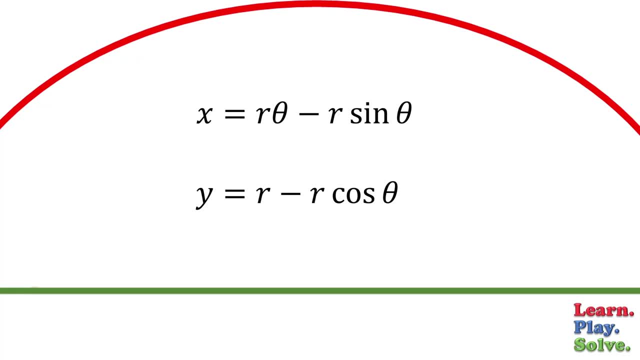 What we want to do is eliminate the parameter theta. This is usually done by solving one of the equations for theta and then plugging that into the other equation. However, if we try to solve for theta with the top one, it'll be impossible. 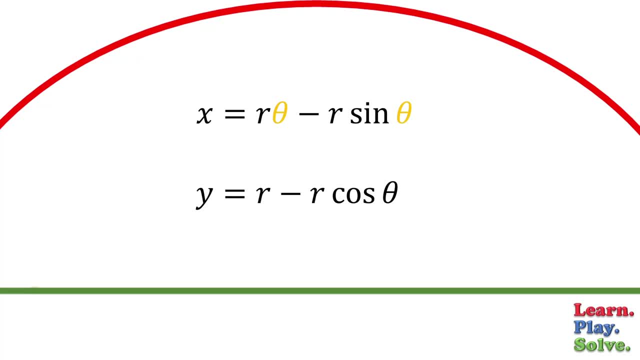 One of these thetas is trapped inside the sine function, while the other one isn't. We can't just factor them out, But we can solve for theta with the bottom one. Just add r cosine to the other side and subtract y. Then divide by r.